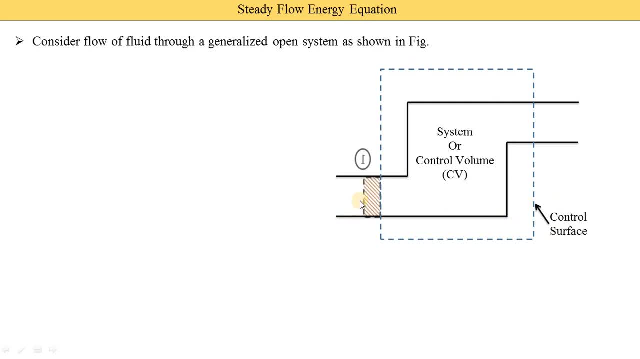 surface Means. on this portion we focus our study. This is the section 1, and this section 1 have a area a1.. Fluid in This fluid have a various parameters: u1, p1, v1, c1 and h1.. Same way at the outlet that we already mentioned. So we move towards the next. 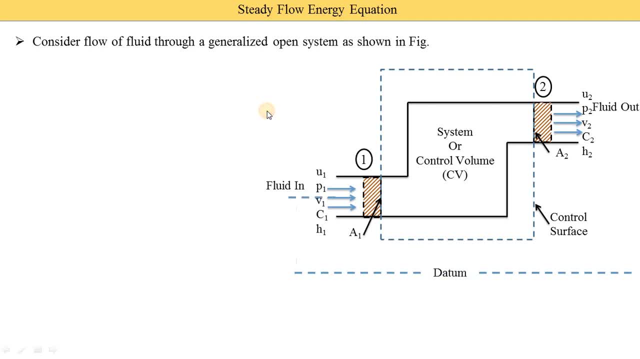 topics. Okay, So next point: The working fluid. enter the system at section 1 and leave the system at the section 2. Passing at the steady rate. Why it is passing at the steady rate? Because the theory name is the steady flow. energy equation Means flow at the steady rate. Flow means that is. 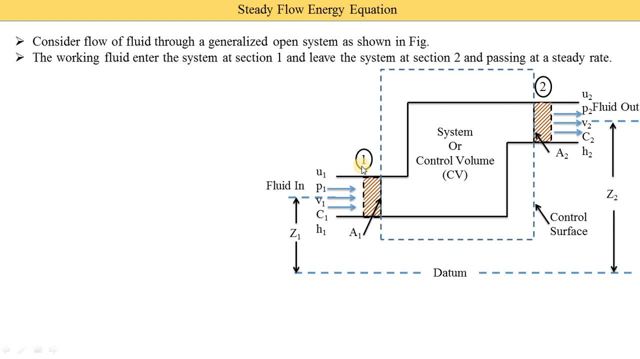 going to change at the steady rate. So the last point is mass out. So let's discuss about the. what is the steady flow and unsteady flow? Okay, So I upload this video today before. If you don't know what is a steady and unsteady flow, then I provide the link on the card. Card means on a top right. 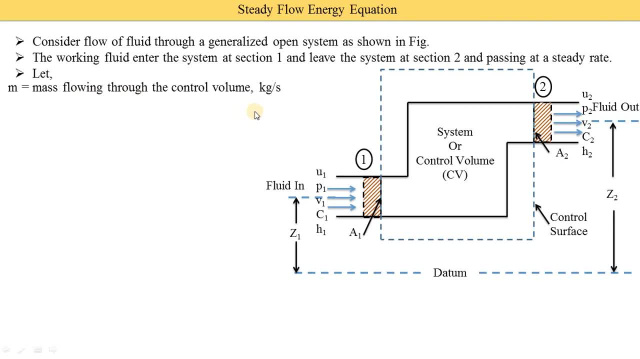 screen of your mobiles or a laptop. you see the I symbols Now. first term is use M. M means that is a mass flowing through the control volume, and the unit of mass is kg per second. Next parameter is kilojoule: okay, but in this image we are not indicating any q and work interactions- okay. 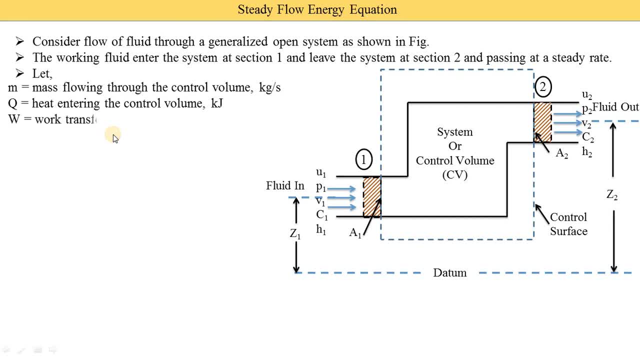 so in every open system it is not necessary. the heat and work interaction is there. okay, suppose we are considered the nozzle, so in a nozzle heat and work interaction is not there. then we consider q and w is zero. okay, so i upload for that all the applications with you later on. 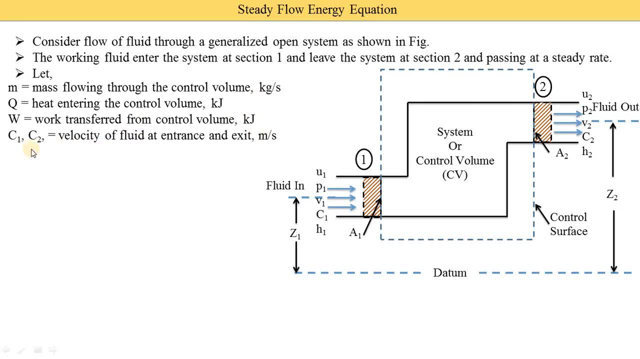 w means work transfer and its unit is the kilojoule. c1 and c2 here. you see we mentioned c1 and c2, so all the one parameter means here. one is written in a subscript. it's indicate the inlet and for the outlet we use the two parameters. so c1 and c2 is the velocity of the fluid at. 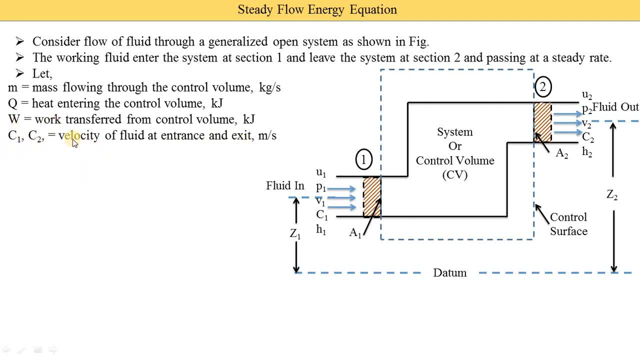 entrance and exit. this c1 is indicate for the entrance, c2 is indicate for the exit in meter per seconds. next one is p1 and p2- pressure of fluid at the entrance and exit, and the unit of the pressure is newton per meter square. u1 and u2- internal energy per kg. 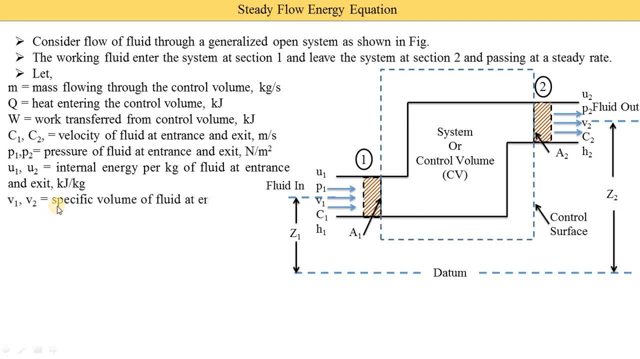 of fluid at entrance and exit kilojoule per kg. next one is the v1 and v2. that is a specific volume of the fluid at entrance and exit meter. cube per kg is the unit of specific volume. h1 and h2: it is the enthalpy of the fluid at entrance and exit. kilojoule per kg- cv. it is. 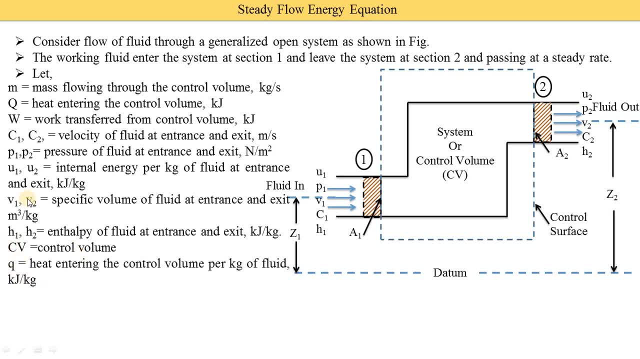 denoted as control volume. now here small q word is used. okay, so already we mentioned capital q. capital q, that is the heat entering. okay, small q is also the heat entering to the control volume, but here per kg of fluid is mentioned. so unit is 10, that is kilojoule. 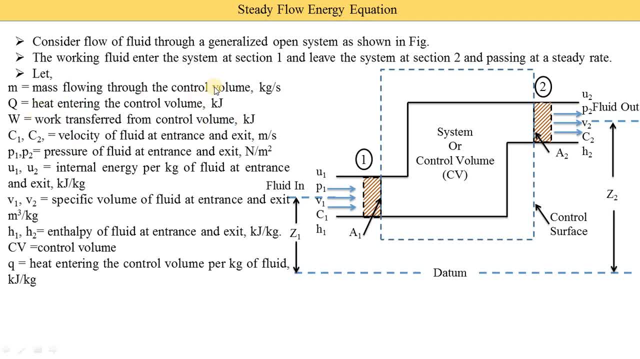 per kg. okay, so here for the, what amount of the mass for this particular mass is given? okay, but when we divide this capital q by the mass, then it gives the small q same way small w that the work transfer is divided by the kg of the fluid supply, then it is converted. 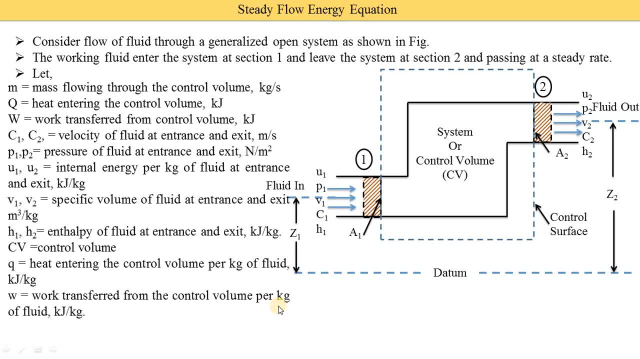 to the small w. that is the work transfer from the control volume per kg of fluid kilojoule per kg. Now we derived this equation for that. okay, one parameter is missing, that is z1 and z2, that is, the elevation of entrance section and the exit sections in a meter. okay, so this: 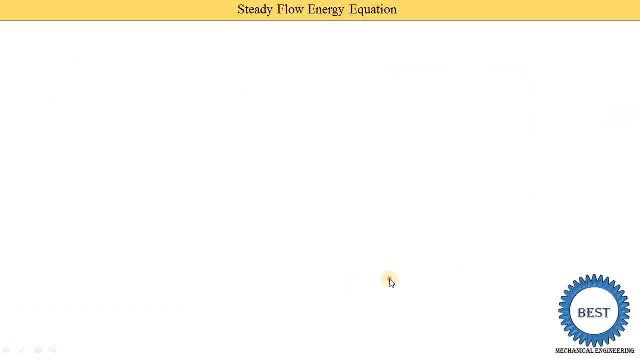 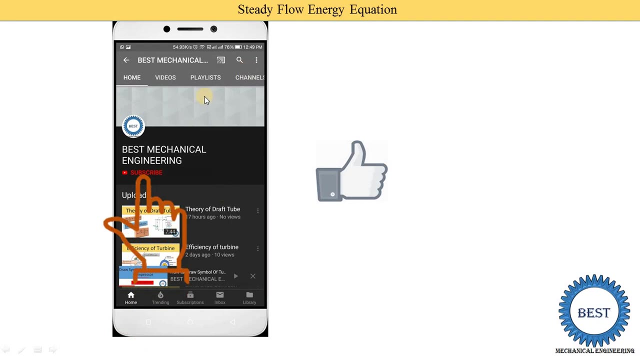 is the one type of the height. it is measured in a meter. now, before moving ahead, I request to like the video and subscribe my channel for watching the more video related to engineering, thermodynamics and another subject of the mechanical engineering for that various playlist is provide. 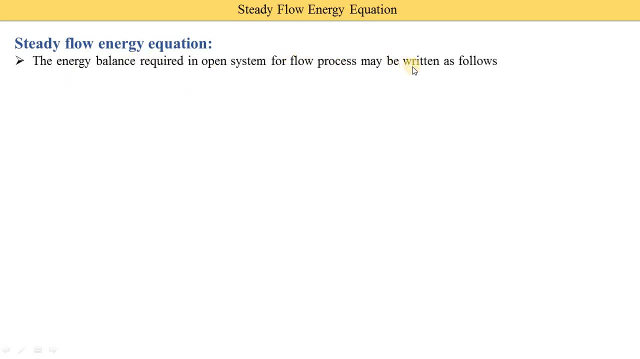 Energy balance required in open system for the flow process may be written as follows. so first we mentioned the energy balance. energy balance means what we supplied and what we get. okay, same way that we, what food we eat, that we measure in calorie and what work we do, that is also converting calorie. okay, then we are balanced. our body is now growing that. 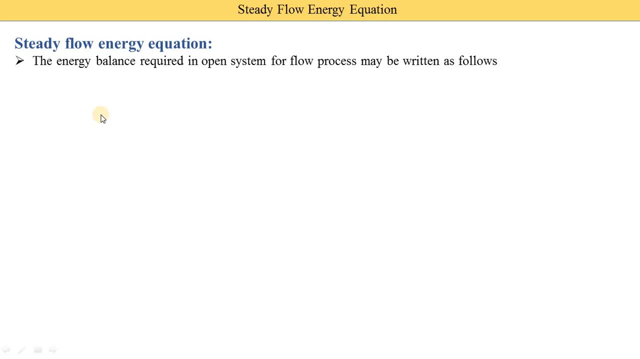 means what we take the calorie from the food is equal to the what work we doing. so same way we applied the energy balance. Okay, Let us now analyze the on the energy balance question to the open systems. okay, so fast. energy enter into the control volume plus. 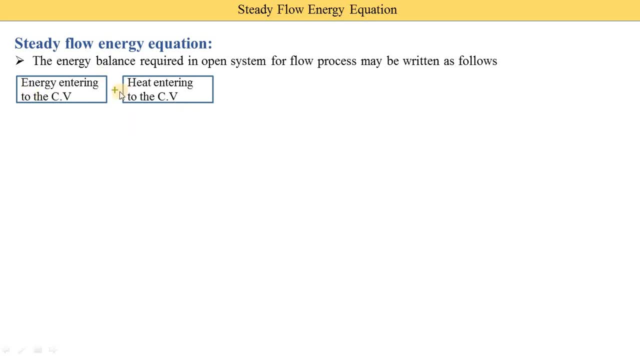 Heat entering through the control volume. okay, so these are the generally to input. There is an energy entering to the control volume plus it entering to the control volume. and what is the outlet? so in our lives there is a three parameters. that is, a energy leaving to the control volume. same way here, energy entered, an energy must be near and suppose. 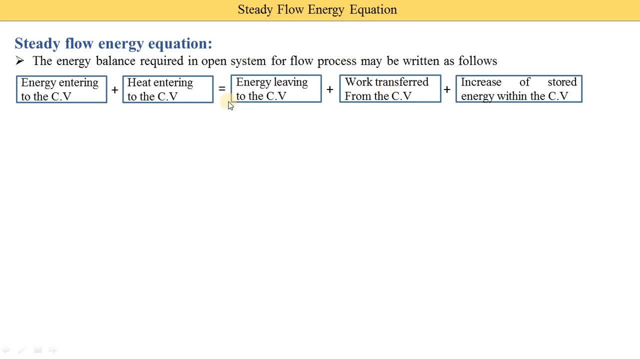 we supplied the heat is converted into the work. and suppose we supplied the work, then we convert in it. convert into the heat, okay, depending on that, we consider here the minus and plus signs, okay, but we consider the heat as a input. same way on the output we achieve some work done. so work transfer from the control. 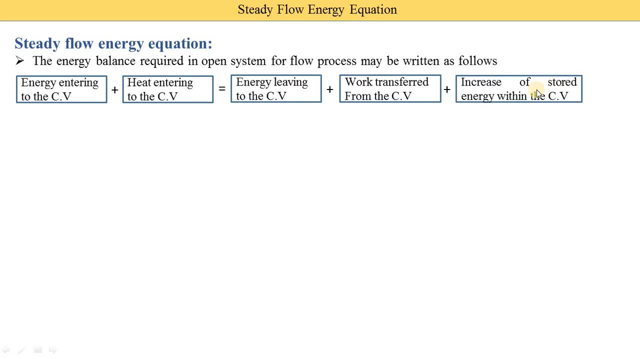 volumes and sometime the energy is store. that is a increase of store energy within the control volume. that's why in outlet, that is a three parameters is mentioned now for a steady flow process. increase of store energy within the control volume is zero means suppose steady flow process means that is a flow is continuously going on, with the constant rates, all the parameters. 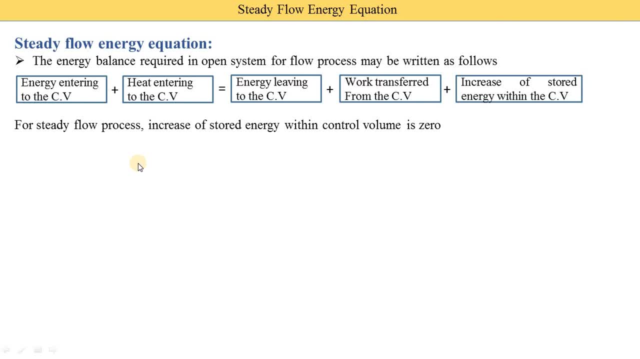 are constant with respect to the time, it is called steady flow process. okay, so when the steady flow process, increase of stored energy means this last term in these above equations are considered as the zero, so only the fourth part is remaining in a inlet, that is, energy entering, heat entering. 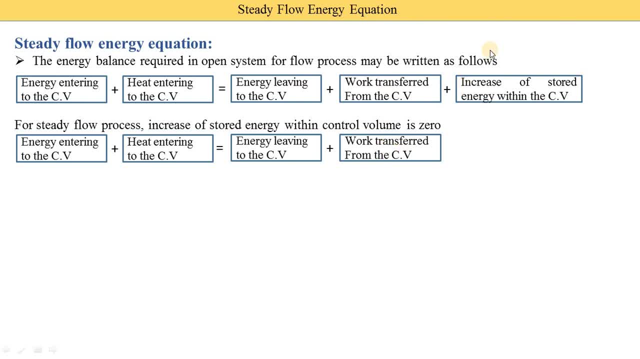 energy leaving and the work transfer from control volume. this parameter is zero for the steady flow process. now this energy entering to the control volume, so that energy in a different forms okay. so it is possible that the internal energy at section one flow work at the section one generally inlet effort, we use the section one okay. 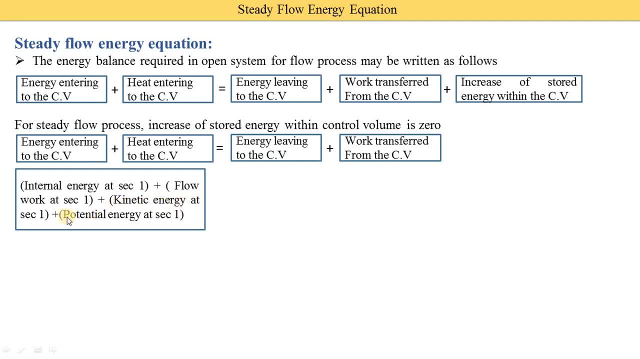 that's why here section one is mentioned. it is also forming a kinetic energy and potential energy- sometimes that is a two or three form of energy- is available. no internal energy is available. so depending on that, we consider the parameter either some value or a zero. okay, second step is: 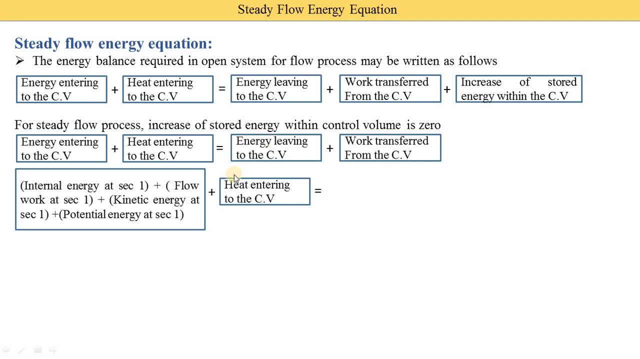 same, that is, a heat entering to the control volume equal to for outlet energy, leaving to the control volume. same way. internal energy at section two. flow work at the section two. kinetic energy at section two. potential energy at section two means it is the same only instead of section one. 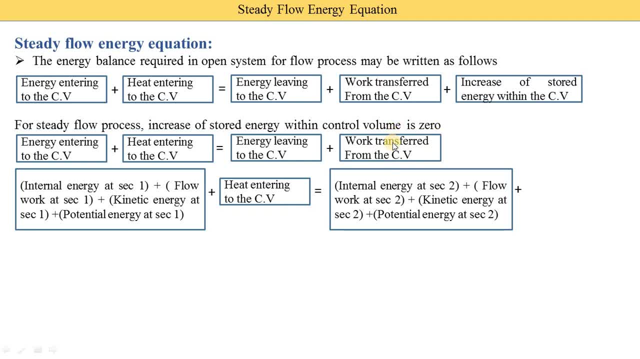 we have written section two plus this parameter is as it is. that is, a work transfer from the control volume. now these things are change in a form of the equations. okay, so we need to these. all the parameters is depend on the mass. okay, if mass is changed and value of this, all the parameters are changed. that's why here it is. 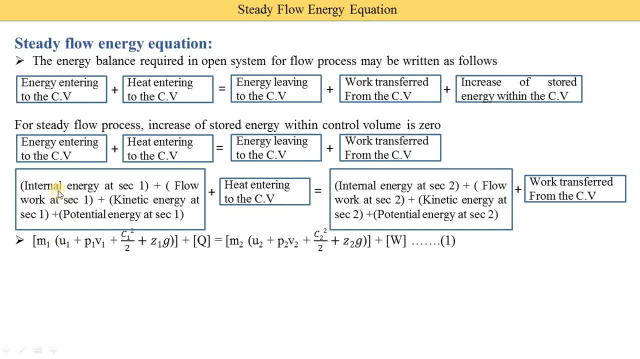 multiplied with the m. okay, so m1 in bracket internal energy is denoted as the u1 flow work. at the section one it is denoted as the p1 v1 kinetic energy. at the section one it is c1 square by two potential energy. at section one it is denoted as z1 into g. 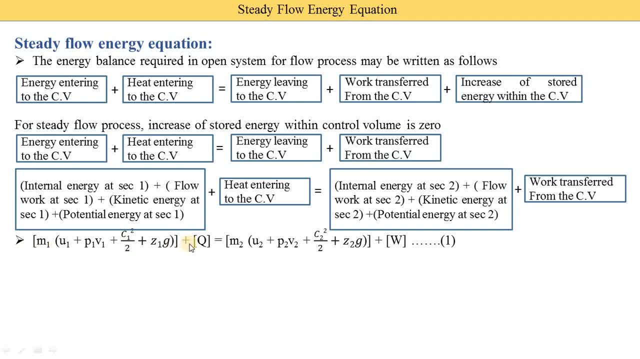 okay, this parameter is over. so we complete this big bracket plus heat. entering to the cv, it is denoted as the q. that we already studied is equal to same way for the outlet. these all the parameters are depend on the mass. so here at the section two means it is denoted as the m2. okay, in bracket. 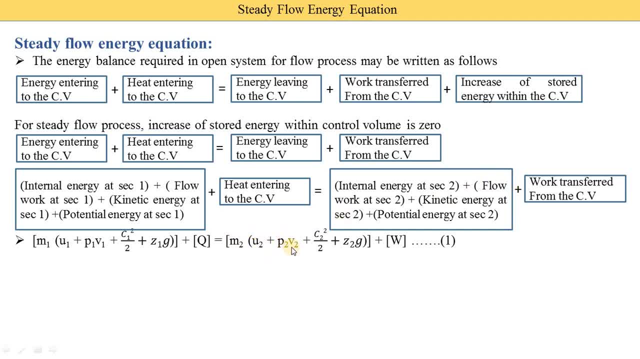 internal energy: u2 flow work. at section 2 it is denoted as p2- v2. kinetic energy: at section 2 is denoted as c2 square by 2. potential energy: at section 2 is denoted as z2 plus d bracket over. 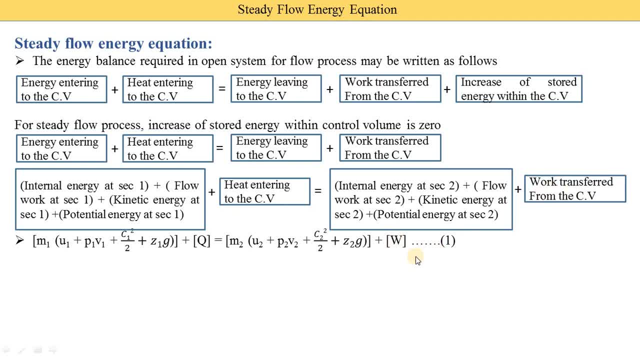 plus word transfer from the control volume. it is denoted as w, so this is the equation number one. okay, so further simplification of this equation is available. okay, from these equations we are deriving the different equations for the different application means for the nozzles for the turbine. 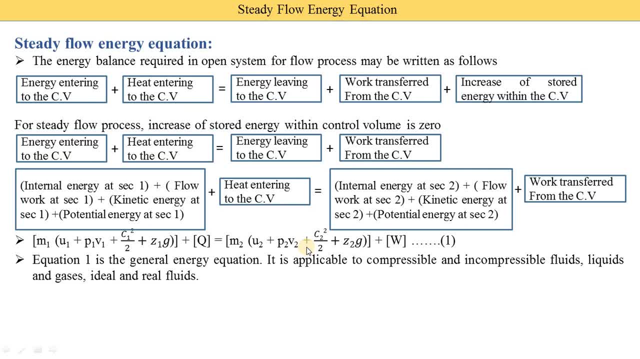 for the pump. that is an equation. derivation is possible from these equations. okay, so i also prepared this all type of the video for all the application that all the videos are available within the week. okay. so equation one is the general energy equation. it is applicable to compressible and incompressible fluid, liquid and gas, idle and real fluids. 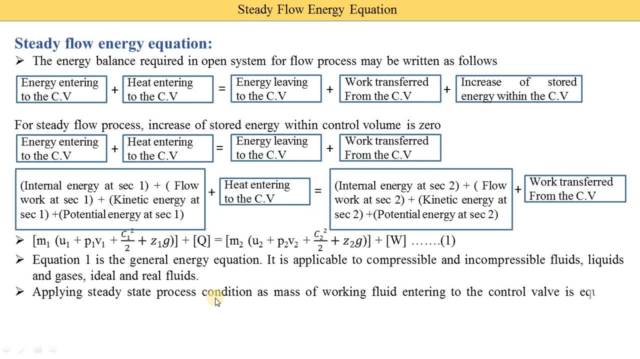 you to compressible fluid, liquid and gas, idle and gas. idle and real fluids. you applying the steady state process condition as a mass of the working flow. applying the steady state process condition as a mass of the working flow entering to the control volume is equal to living from the control volume means. 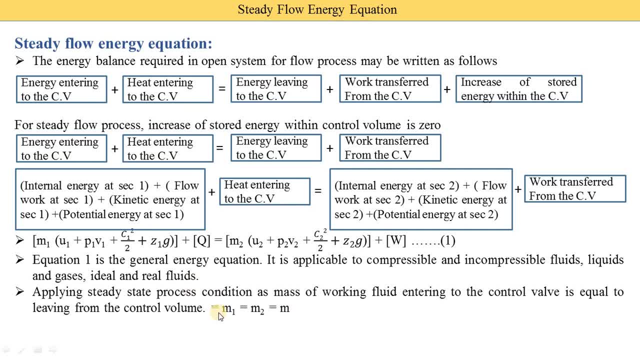 m1 is equal to, m2 is equal to m. so we consider the steady flow means mass is flowing at constant rate. so m1 is entered, then m2 is living. okay, so both have the same because it is the steady flow process. so it is m 1 and m 2 are replaced with the m. 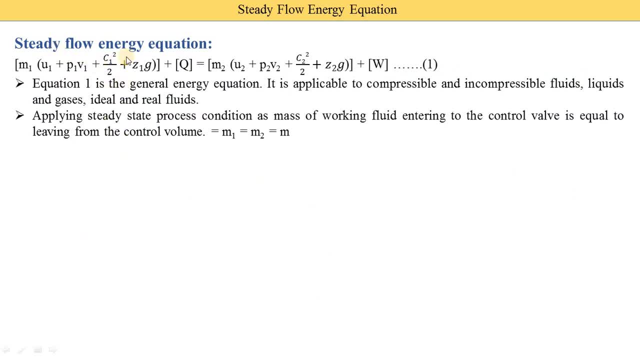 called a further calculation. okay, so i taking this same step again. okay, so here from the the next step. so we replace this m1 as a m and m2 as a m. okay, solder parameters are same. we are not changing any things now. this u1 plus p1, v1 means internal energy plus flow. work is denoted as the. 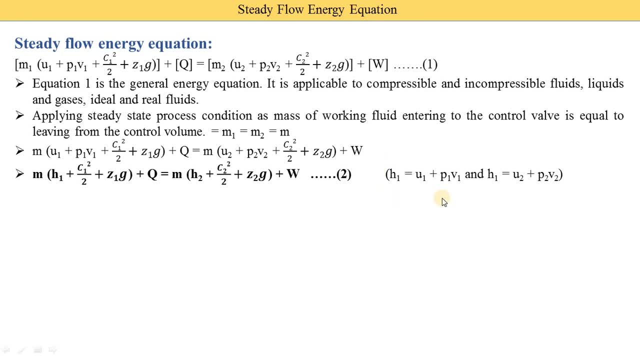 enthalpy. so here you see that u1 plus p1 v1 is written as the h1. u2 plus p2 v2 is replaced by the h2 here by mistake. the h1 is there, but it is h2, okay. so here you see that the u1 plus p1 v1 is. 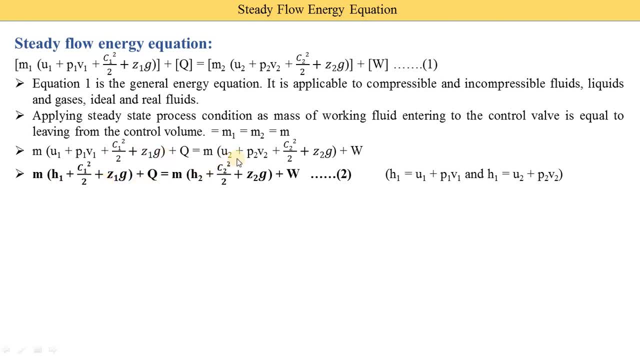 replaced by h1. another thing is same. same way here u2 plus p2, v2 is replaced by h2. other parameters are same. so we consider this is the equation number two. equation two is called a steady flow energy equation and this is also the first law of thermodynamics applied to open system for steady 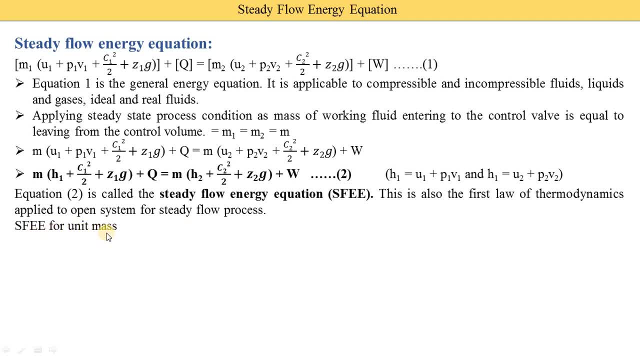 flow process. steady flow energy equation for unit mass. as f double e means it is a short form of steady flow energy equation. now for unit month means we need to divide this equation by the mass. it is called as the unit mass. okay, so we divide these all the parameters by the mass. so here with this, 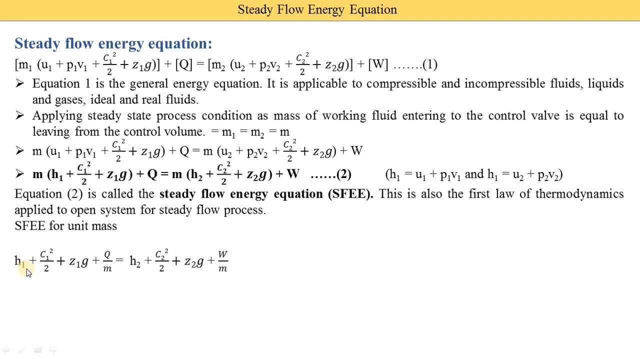 parameter m is already there. okay, so this m is cancelled. so h1 plus c1, square plus z1g. with this q, m is not in multiplication, so we need to divide. so here the we divide the q by mass. same way here, with all these three parameter, m is dead. so we divide by m, so m is cancelled. so 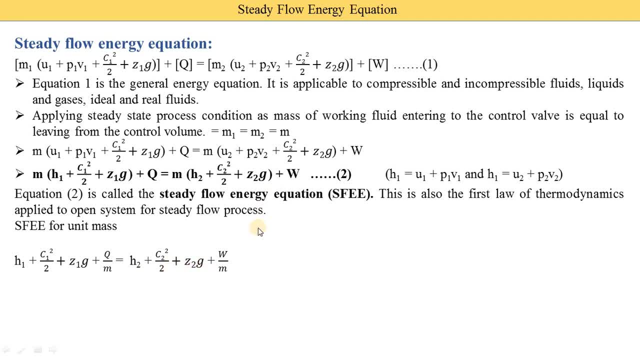 f2 plus c2, square plus z2g plus work, then divided by m: okay, that is a w by m. so we already study in the notifications that the q by m is written as the small q and work, then w by m is denoted as the small w. okay, so these equations are changed. other parameters are: 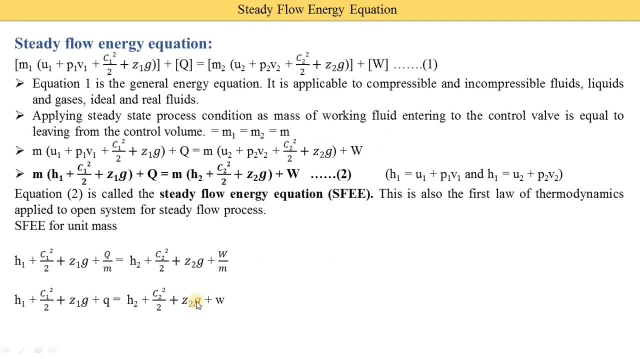 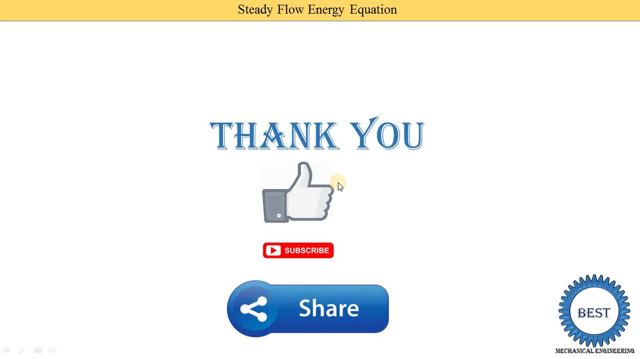 remains constants. so this is the final equations, but generally we use these equations- that is equation number two, for the further application means deriving further, further equations. so thank you for watching this video. if you learn something, then like the video. subscribe my channels and don't forget to share. with your friends.